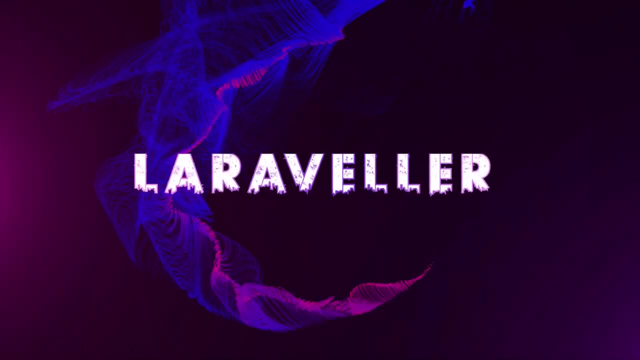 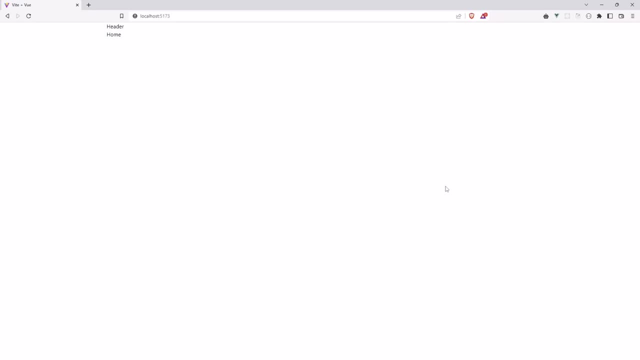 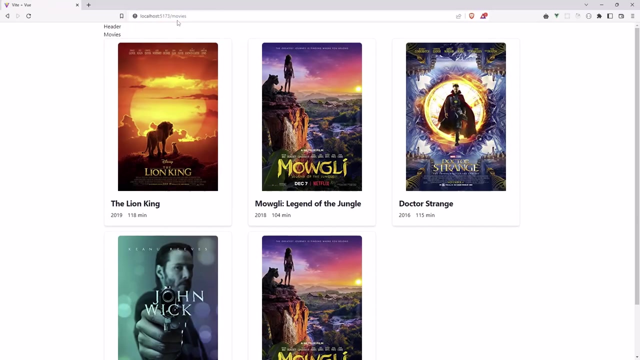 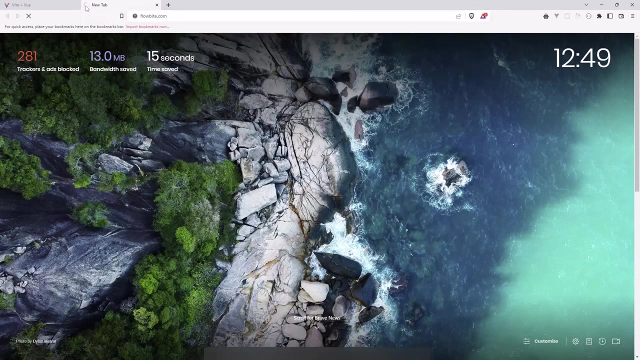 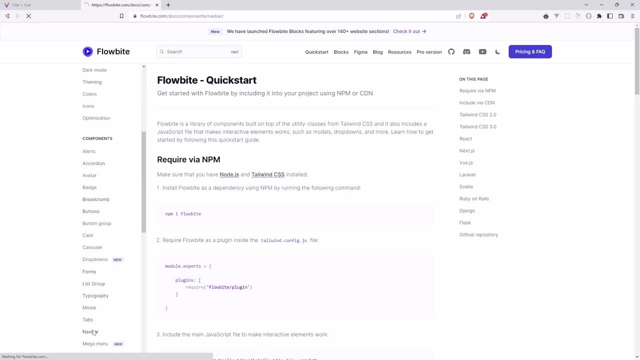 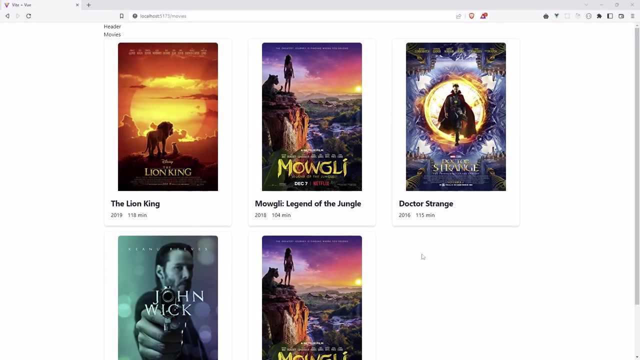 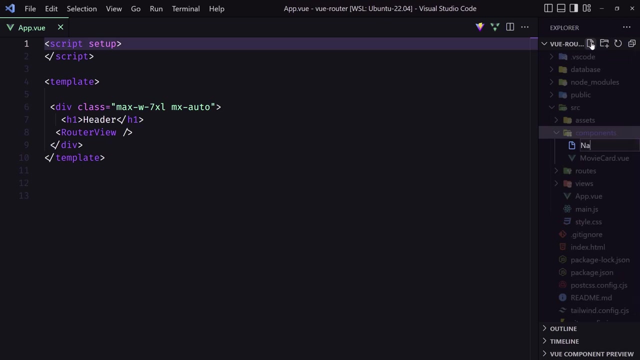 Hello friends, welcome In this video. I'm going to add the navigation here, because right now, if we want to go to the movies, for example, we need to write here movies and let's go. Okay, So for that let's open the flow byte And I'm going to copy the navigation from here. So let's go to the navbar And let's copy this, the first we have here- close, open the VS code And inside the components I'm going to create a new one And I'm going to name it navbar. 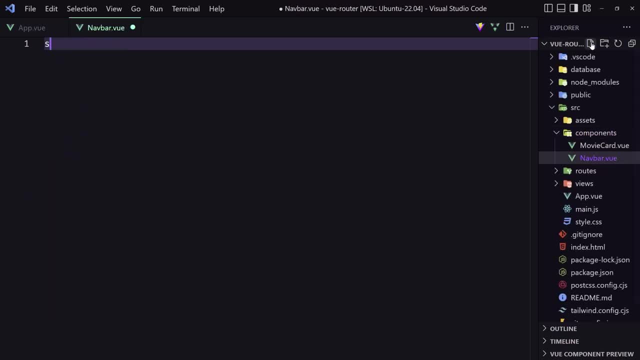 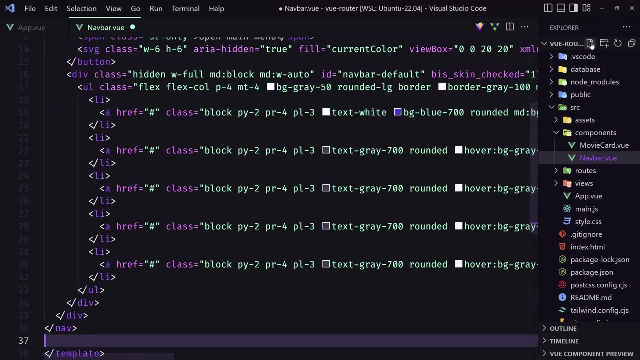 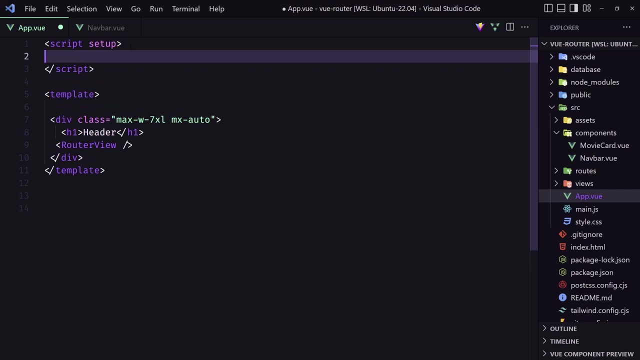 view. Create the view setup here, v setup, And in the template let's paste what we have to copy: save. Now go to the appview. import this navbar component we created. So let's import that Navbar and not navbar view, but just navbar. And inside here now let's: 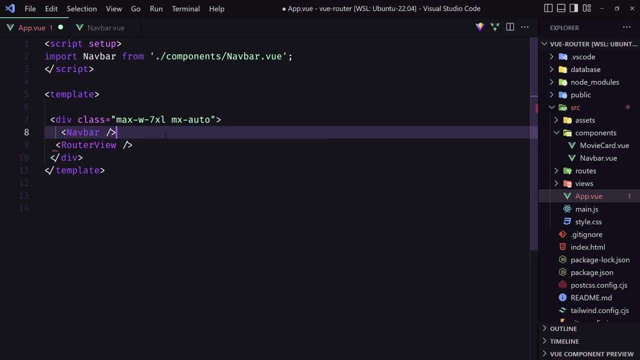 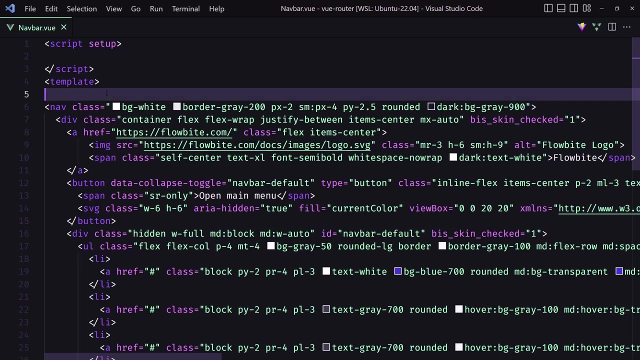 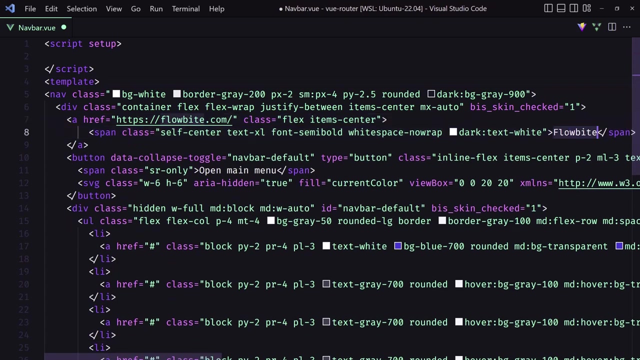 add the navbar. So close this, save. And if we see now, yeah, we have the navbar, Let's make some changes first in the navbar. So I'm going to close this, close the files here because it's too large. First I'm going to remove the logo And then here I'm going to say: view router. Okay, that's it. 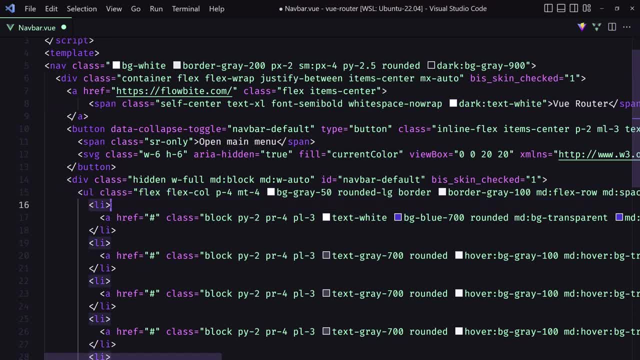 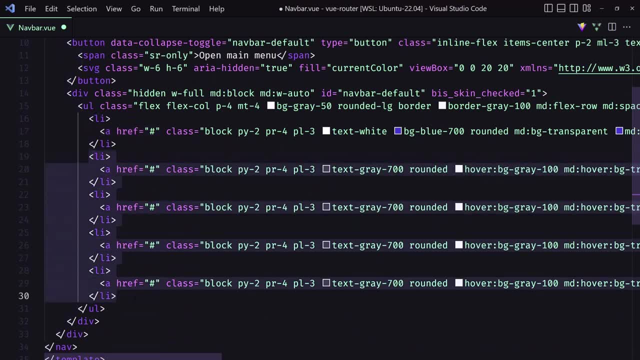 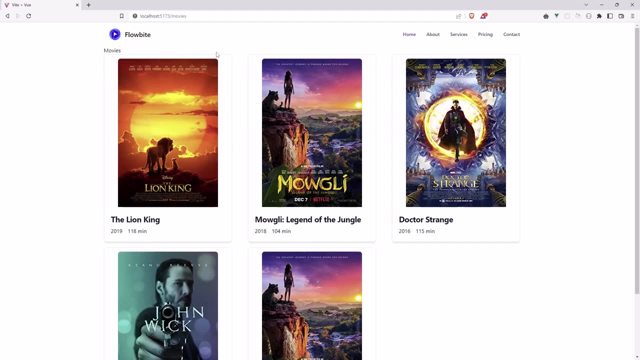 And then we have the ul with the li And here we have the anchor tag I'm going to remove. I'm going to leave only one and remove the others. And here we are not going to use the anchor tag because the anchor tag is going to reload the page And we don't need that. we need to because we have a single page application. we need to go and not reload the page. For that we are going to use the router link. So let's say here: 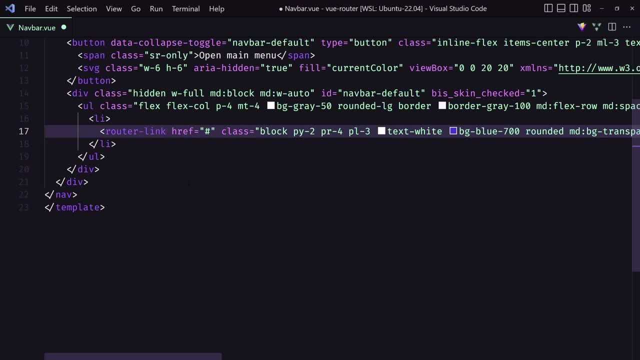 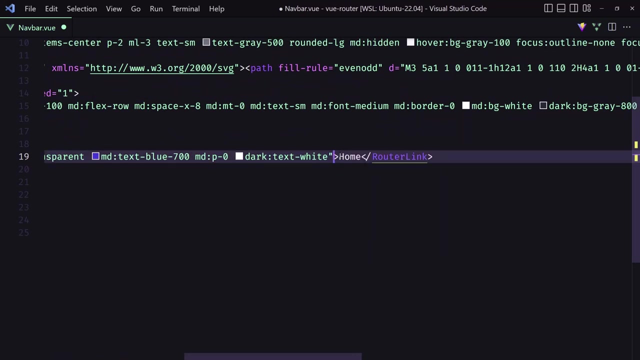 router link like this, or you can use the router link like this if you like, and here we need to say router link to the slash to go to the home page, because here we need to go to the home page. and let's me indent like this, because the fonts are too big for you. 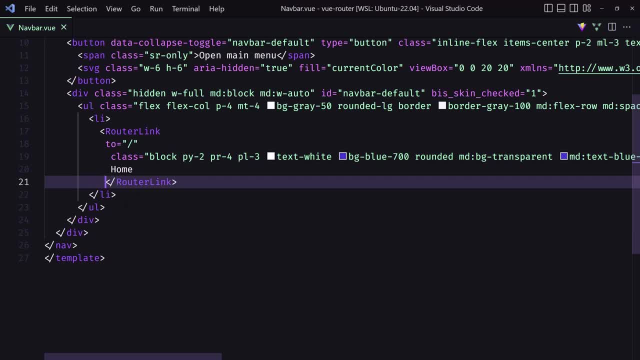 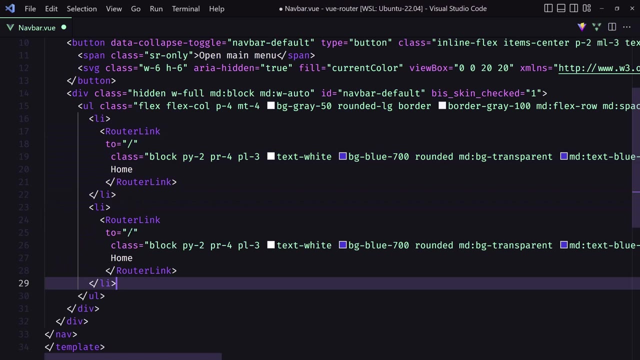 and i'm going to do something like this and if i save and let's go and see, yeah, we have this home. and if i click we go to the home. now let's add the link for the about and for the movies router link to them about. so slash about. here we need to say about. 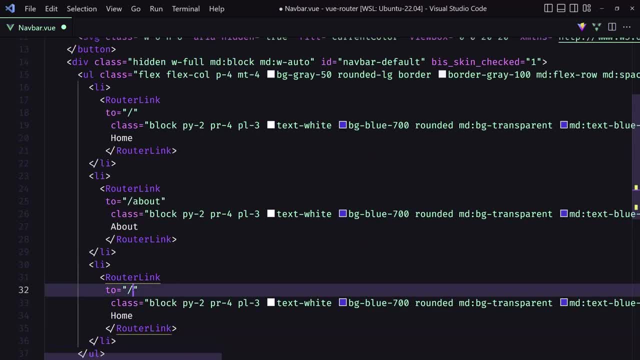 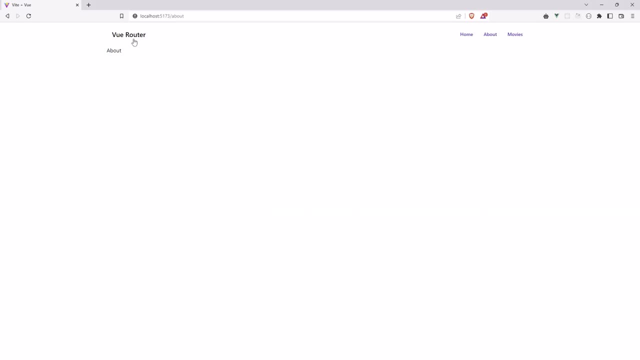 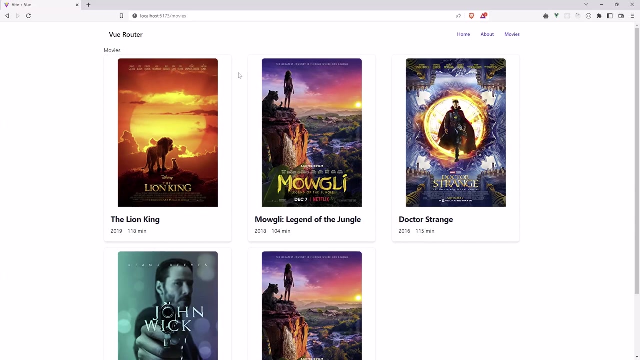 and the last is for the movies. let's say sash movies, and here we need to say movies as well. save, we have home about movies. let's go to the about. we add ins. we are inside the about. let's go to the movies. yeah, we are here and, as you can see, if we go here and 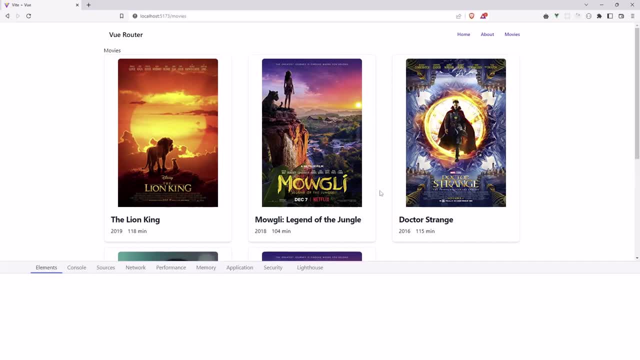 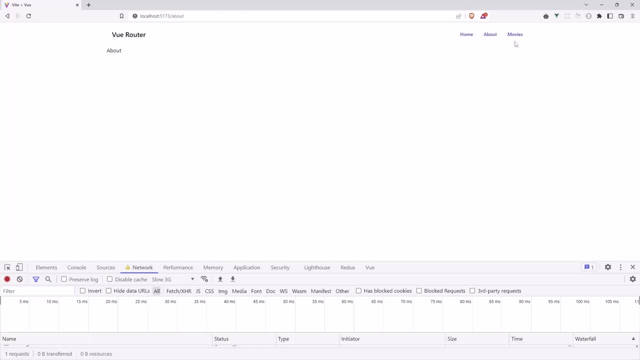 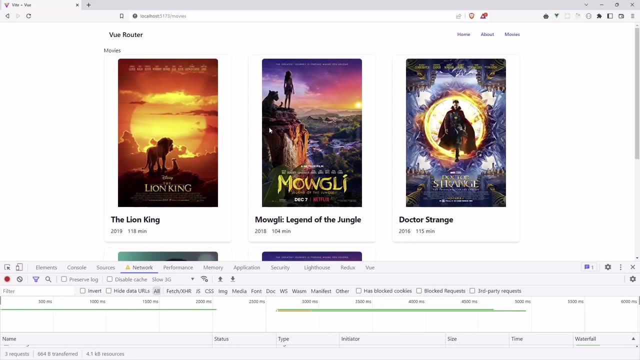 navigate back to the movies. let's just inspect the elements, go to the network and slow 3g here. let's go to the about and now go back to the movies i have. as you can see, it's going to take some time to get the movies because it's going to make the api. for that, let me. 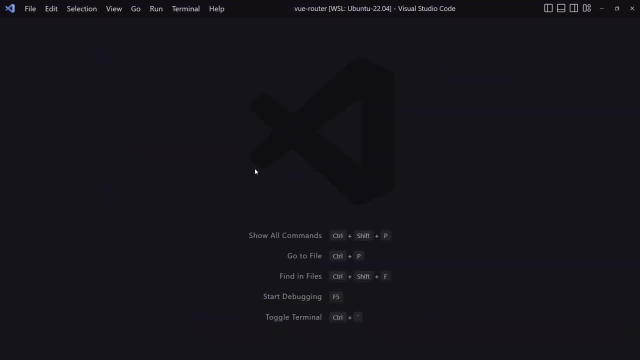 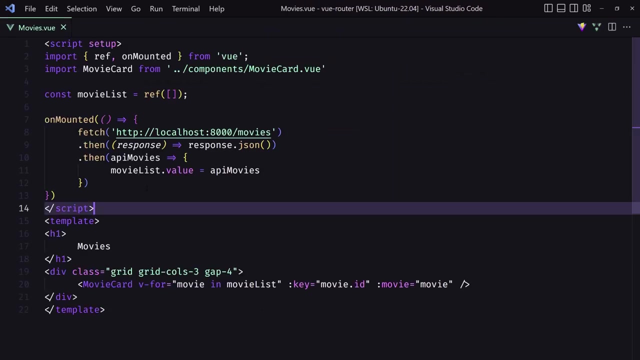 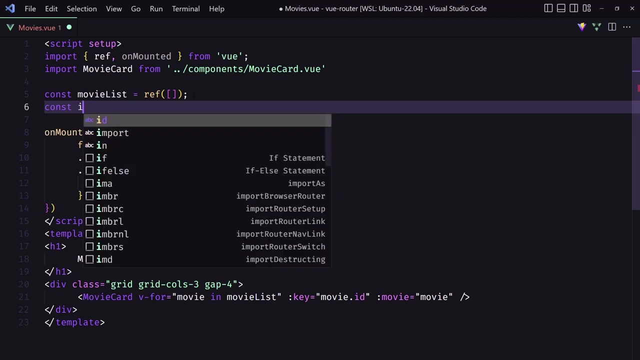 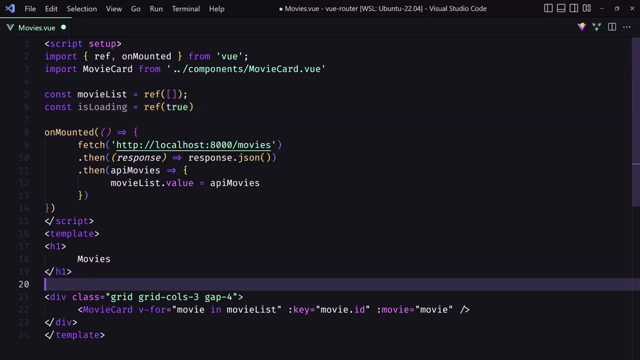 just close this and open the movies view. and here i'm going to create a ref. so let's say const, i'm going to say is loading, loading to be a ref and by default is going to be true, very good. and down there now i'm going to say a div with a class max, with the b small mx. 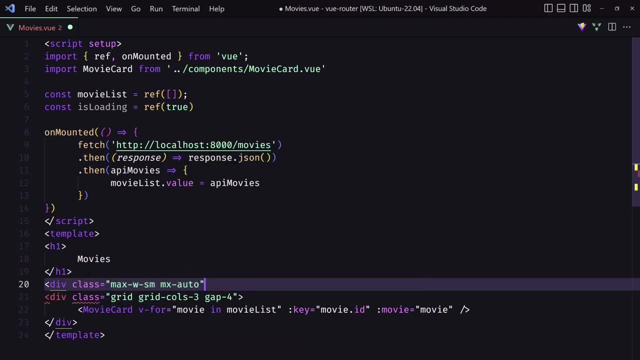 auto and here i'm going to add a span with the class, let's say text to excel and font bold, and I'm going to add text, maybe indigo, indigo 700, like this and let's say: is loading dot, dot, dot. okay, if I save now and let's see. 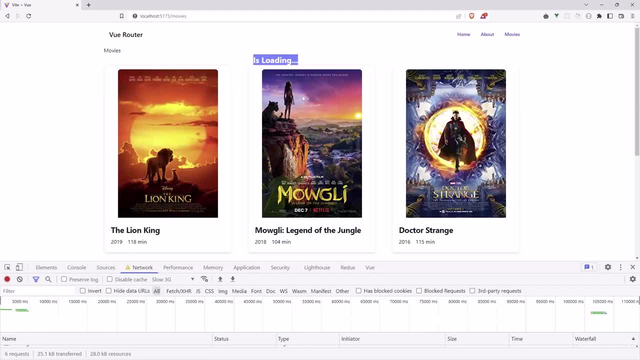 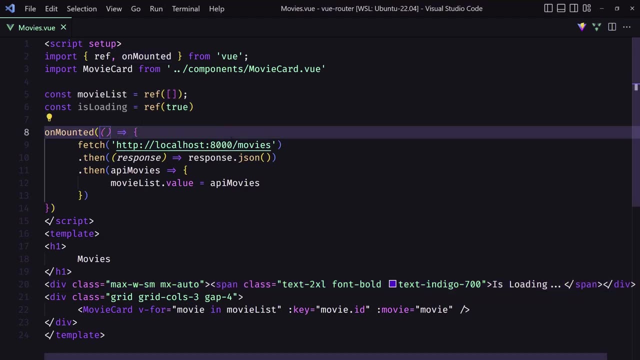 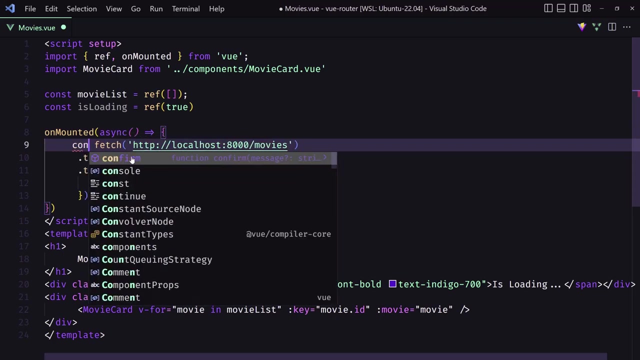 yeah, we have this is loading here, very good, but I don't want to show. this is loading all the time. I want to show only when we don't have movies. so for that, I'm going to make this an async function. first let's say async, and now I'm going to create a constant. 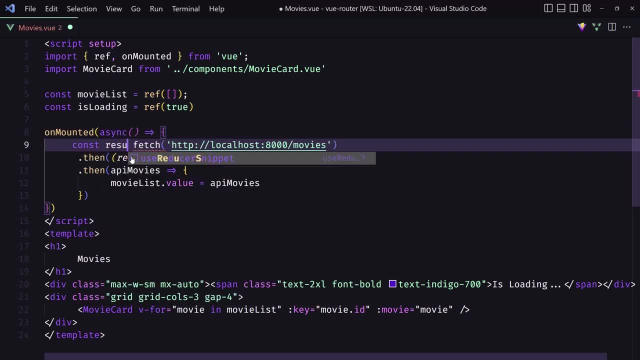 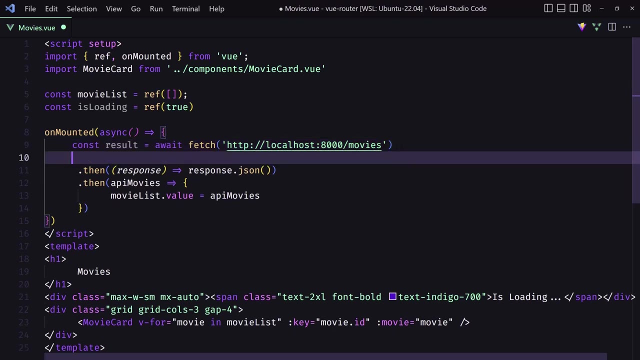 for the result, which is going to be people with await catch movies. okay, then I'm going to create also a constant, another constant, and say response, which is going to be equal with await and response, resultjson, resultjson like this, and then let's remove what we have here. 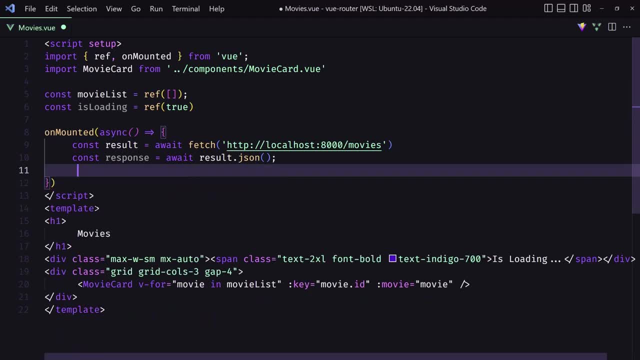 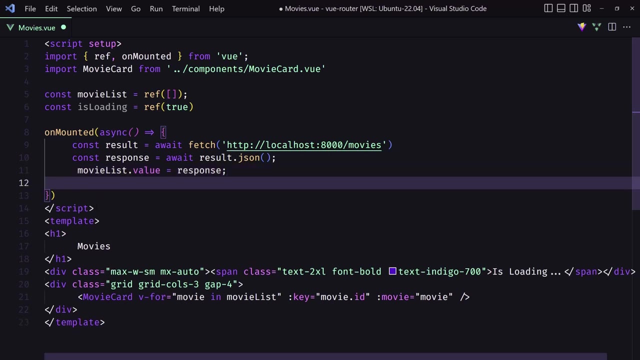 then I'm going to say: the movie list dot value is going to be equal with the response we get. and now I'm going to change the value of this response, that isLoadingvalue, to be false. Okay, and right now, here I'm going to say I'm going to show this isLoading only if this isLoading is true. and let's say: